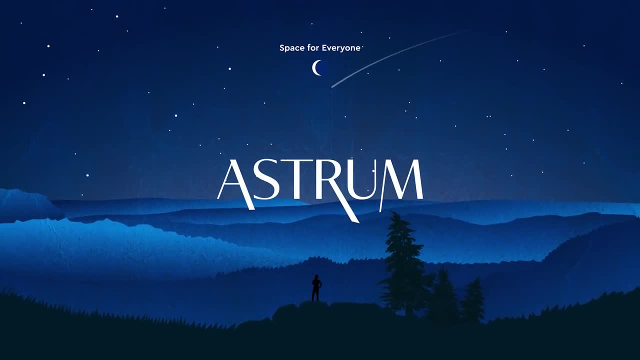 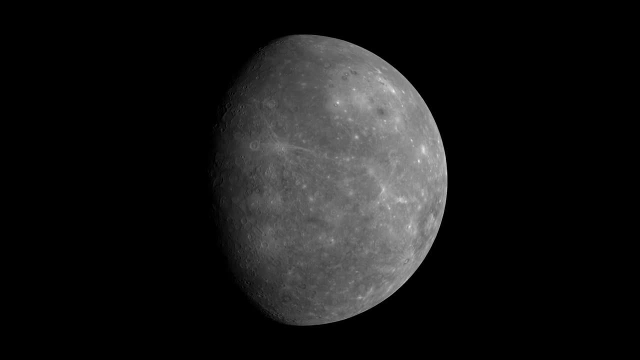 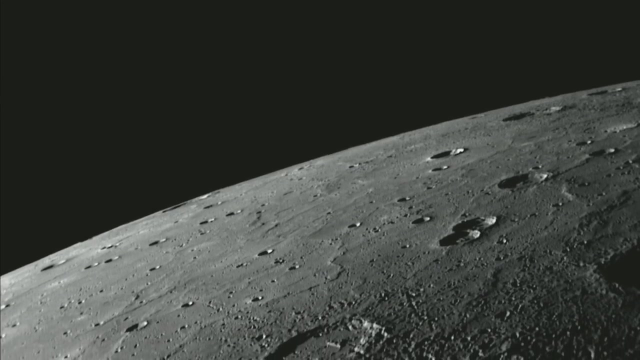 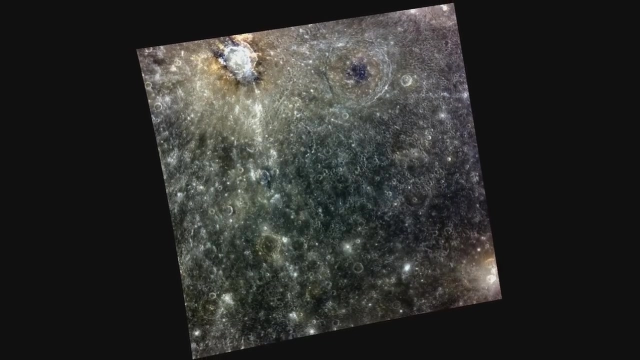 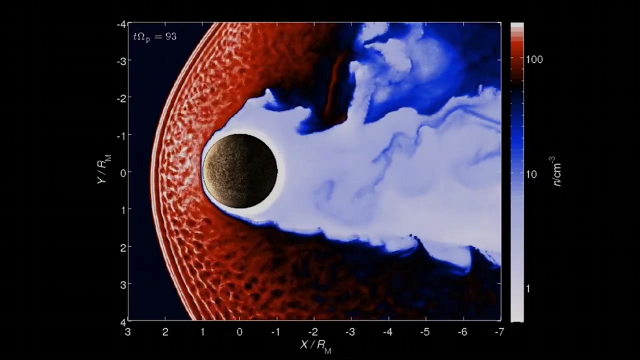 Mercury, the solar system's closest planet to the Sun. Everything I'll show you today will be an actual picture or video image of Mercury from the MESSENGER probe. We'll discuss Mercury's orbit and rotation, its physical characteristics, its surface conditions and the magnetic field and magnetosphere of the planet. 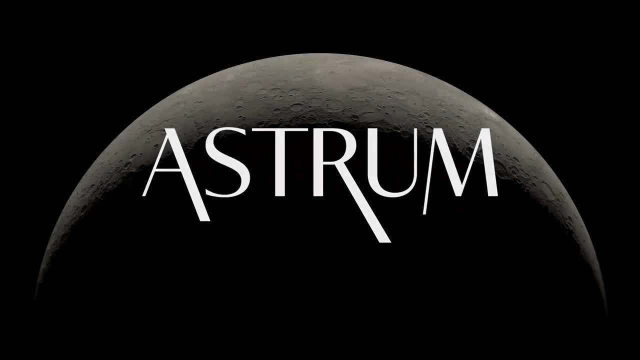 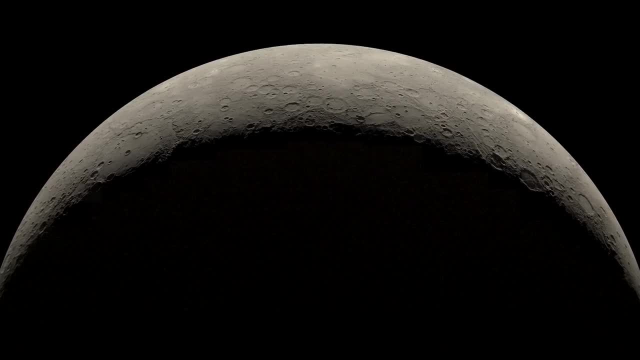 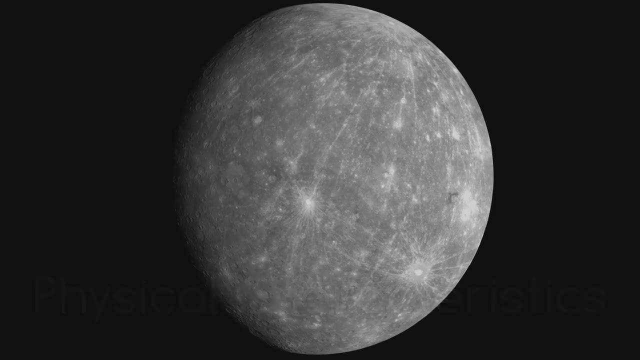 I'm Alex McColgan and you're watching Astrum. Stick with me on this video and you will learn almost everything you could want to know about this tiny yet fascinating planet. Now, when you think about the physical characteristics of Mercury, I'm sure you imagine it being. 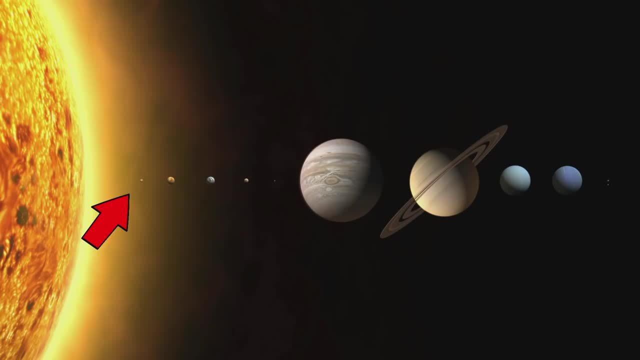 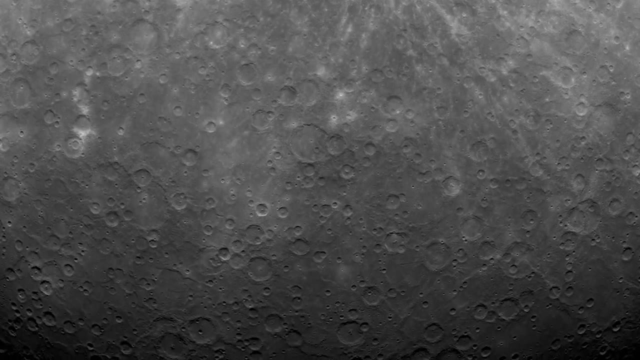 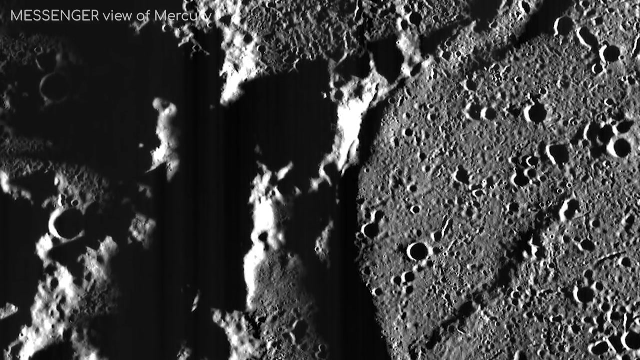 the closest planet to the Sun, but also that it's this giant rock. You wouldn't be too far wrong with that. but it is much more interesting than what you may first think. For example, when I look at Mercury, I do think of our Moon, but Mercury 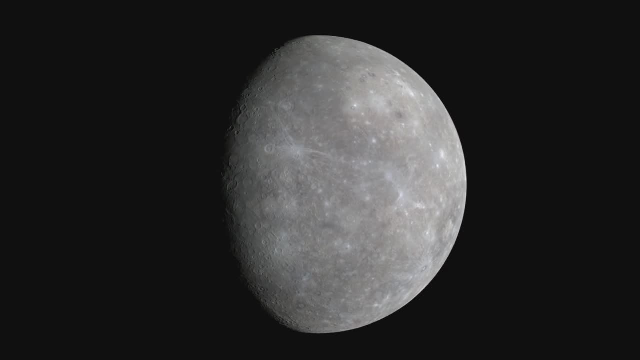 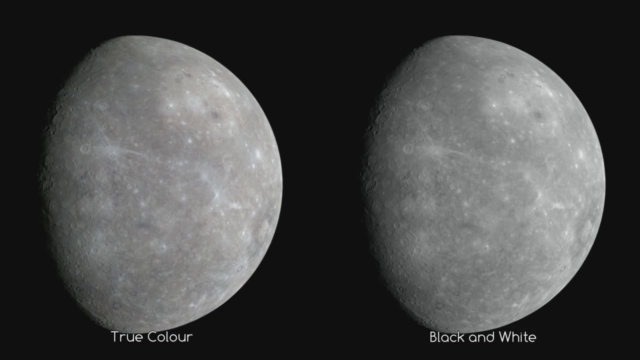 actually is visually more appealing than our Moon. Look at it in its true colour. The first thing that I notice is that it actually does have a colour. it's not just different shades of grey And what else. Well, did you know? for example, 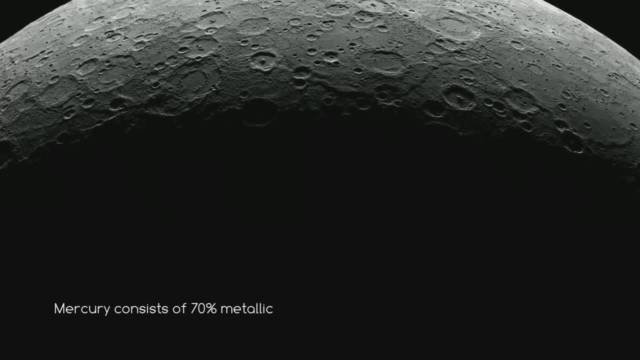 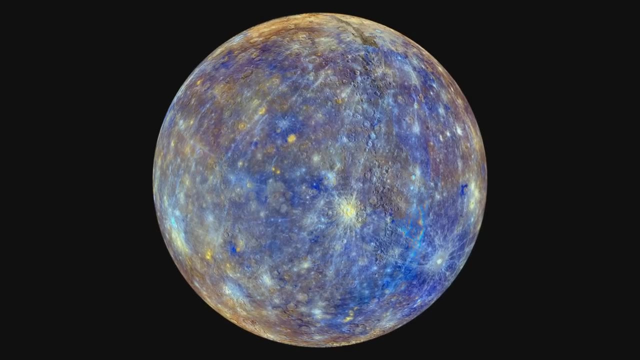 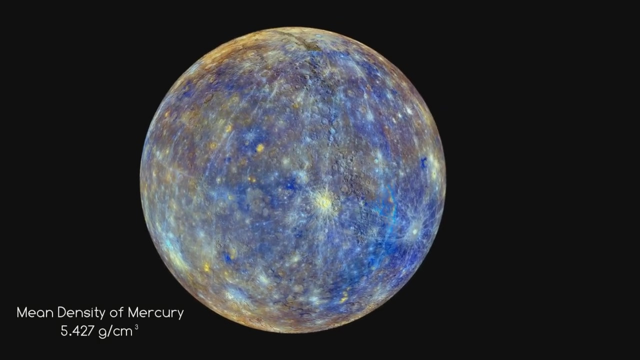 that Mercury consists of approximately 70% metallic and 30% silicate materials, So it's actually more metallic than rocky. Because of this, Mercury's density is the second highest in the solar system, at 5.427 g per cm3, only slightly less than the planet with. 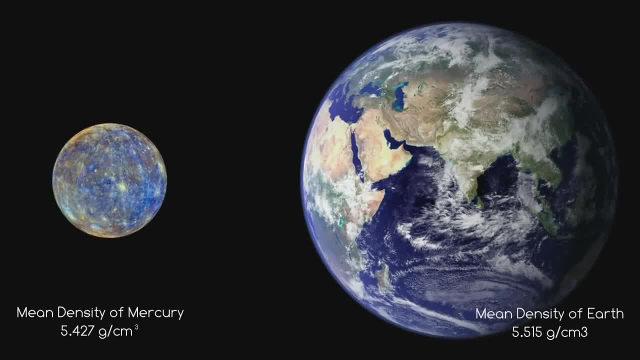 the greatest density, that of Earth, at 5.515 g per cm3.. If Mercury happened to be the same size as Earth, that would mean it would be the largest planet on the planet. and that would mean it would be the largest planet on the planet, and that would mean it would be the largest planet on the planet, and that would mean it would pretty much have the same gravitational pull at its surface. But being the size that it is, its surface gravity is only 3.7 m per second squared. If you were to compare its gravity to Earth, it would look something. 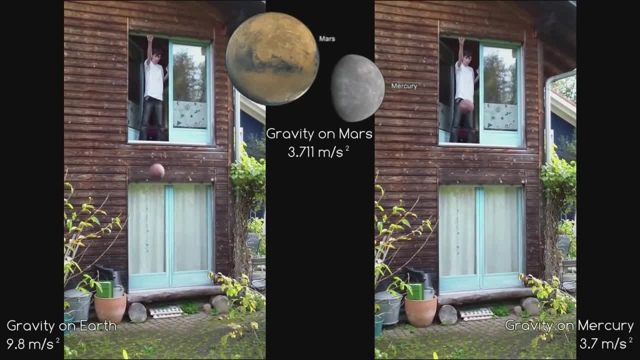 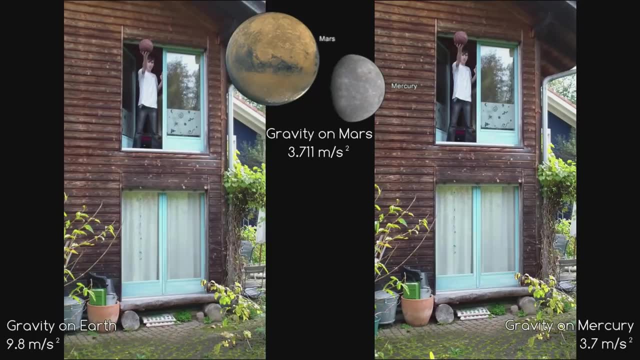 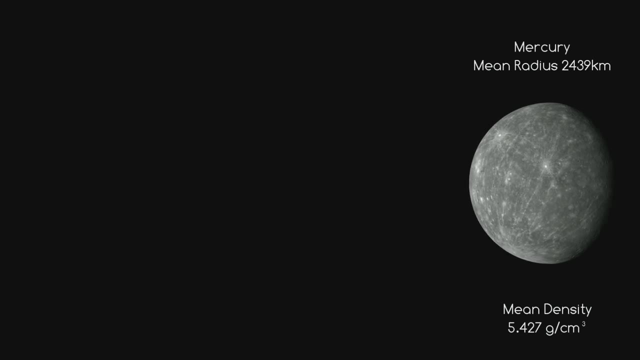 like this. This means the surface gravity of Mercury is only slightly less than what it is on Mars and considering that Mars is a much bigger planet, that just says something about the density of Mercury. But before we leave the subject- here's subject- of Mercury's size. I want to show you one last comparison, that of Ganymede. 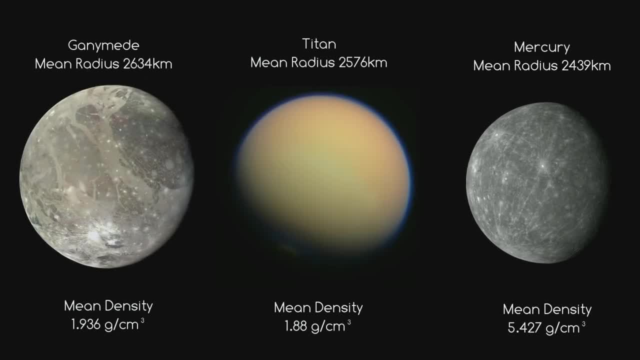 and Titan against Mercury. Now, Ganymede is the solar system's biggest moon and also the biggest moon of Jupiter, while Titan is Saturn's biggest moon and the second biggest moon in the solar system. These two giant moons are bigger than Mercury, as you can see. 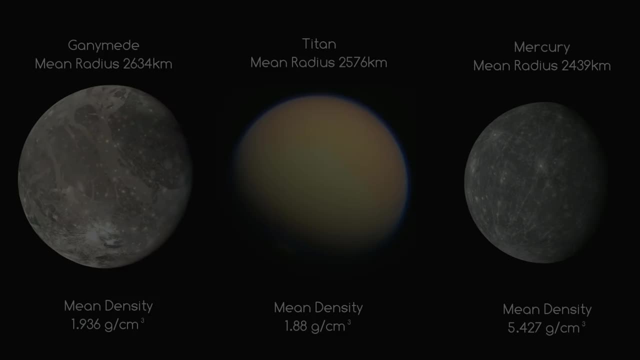 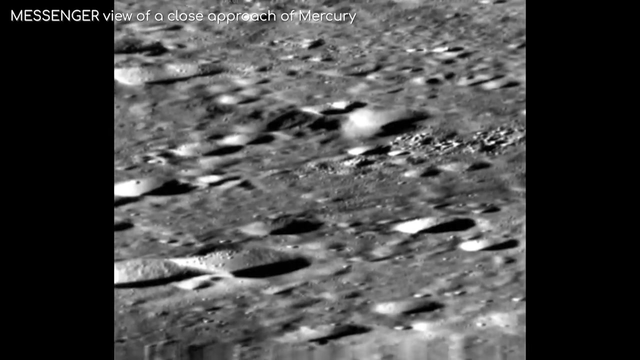 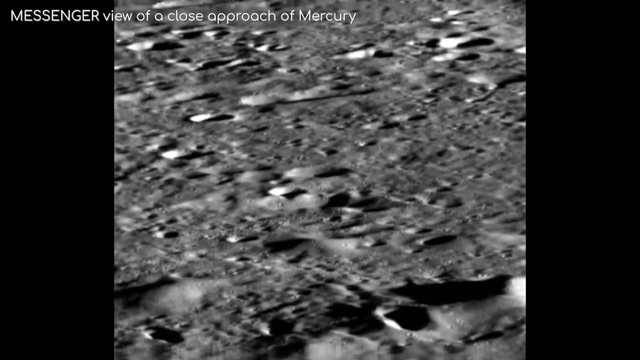 here, but their masses are far less. If you look closely at Mercury's surface, you'll see its appearance is similar to that of our moon. It shows extensive mare-like plains and heavy cratering, indicating that it has geologically been inactive for billions of years. But it obviously was geologically. 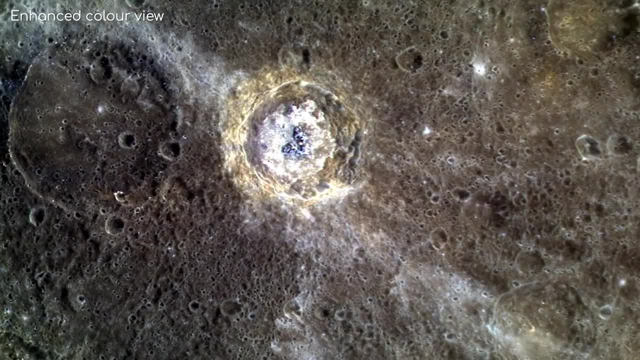 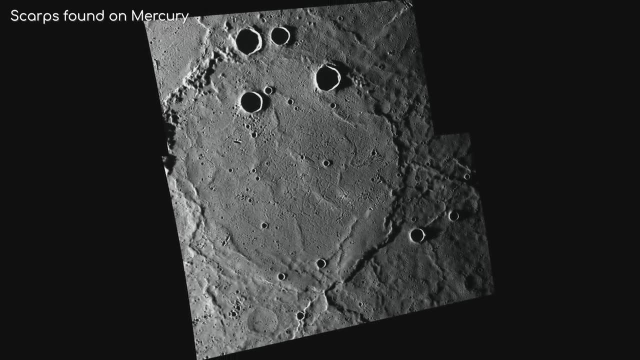 active at one point, because one of the distinctive features of Mercury's surface is the presence of many narrow ridges extending up to several hundred kilometres in length. It's believed that these were formed as Mercury travelled through millions of miles of galaxies to form 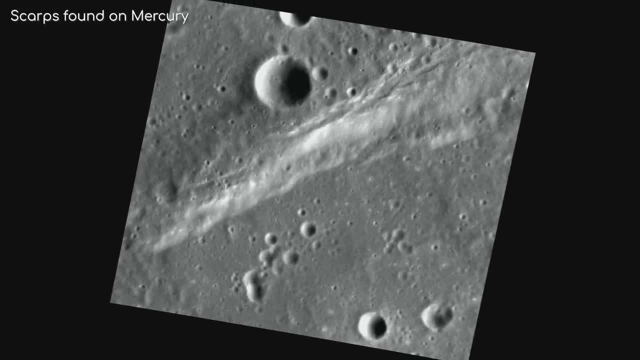 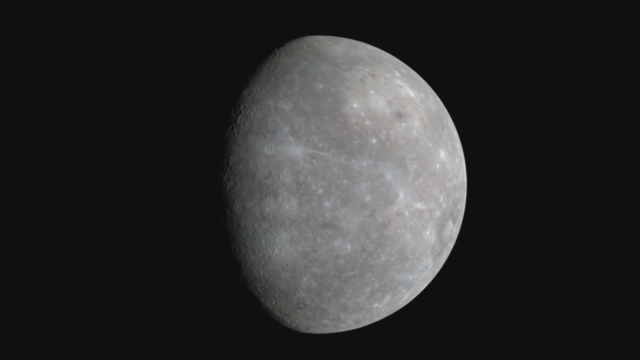 Apollo's orbit. Mercury's core and mantle cooled and contracted over time when the crust had already solidified, And one of the most distinctive things you'll notice about Mercury is this huge crater on its surface called Caloris Basin, with a diameter of 1,550km. 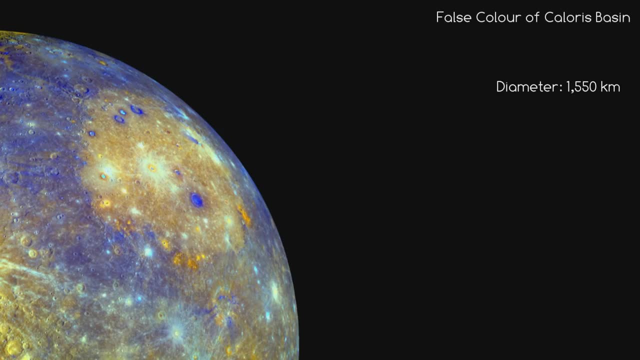 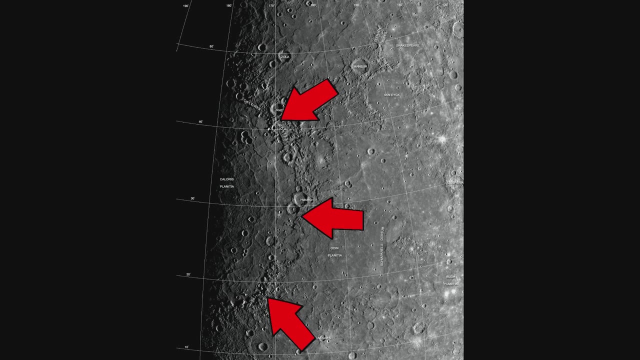 The impact that created Caloris Basin was so powerful. it caused lava eruptions and left a concentric ring over 2km tall surrounding the impact crater. At the antipode of Caloris Basin is a large region of unusually hilly terrain known as. 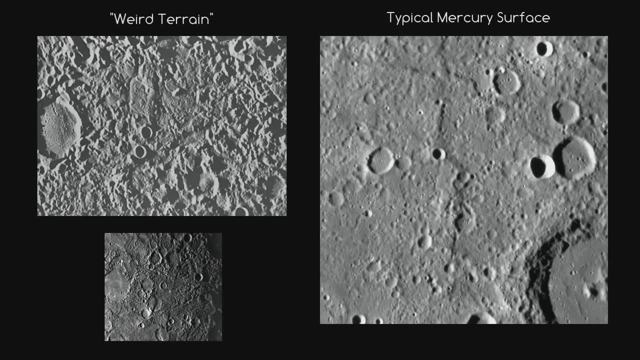 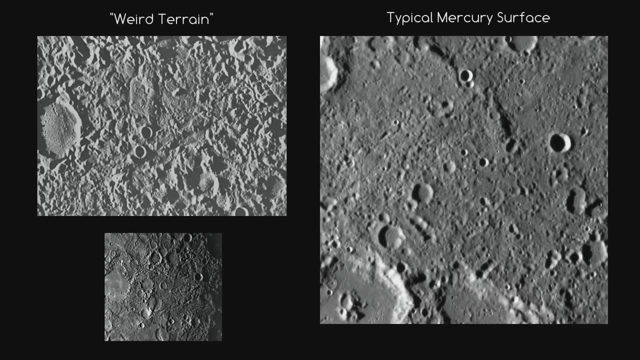 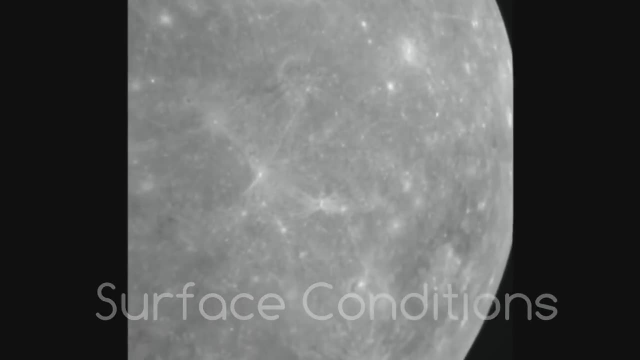 the Weir's Terrain. If you compare this region to the rest of Mercury, you can see why it would have this name. So what's it like on the surface of Mercury? Well, to start with, the surface temperature is hugely different all over. 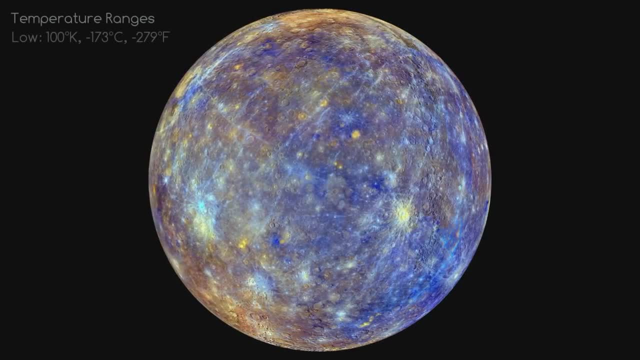 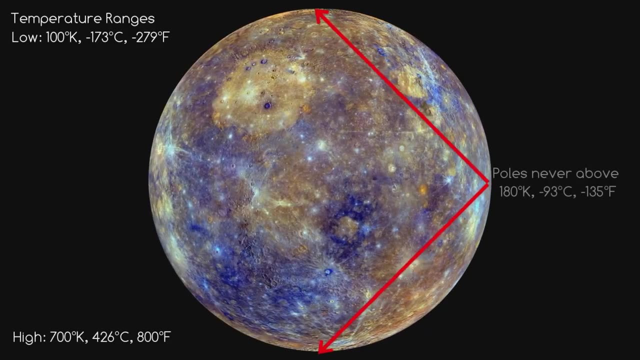 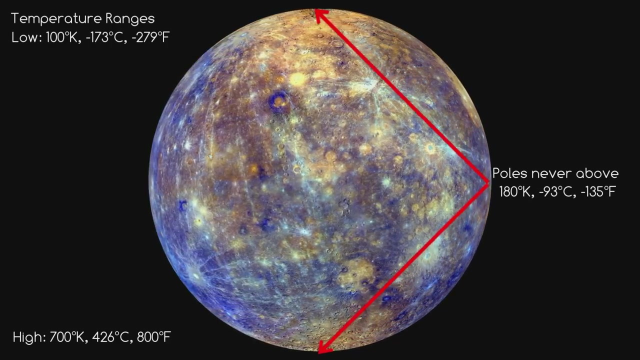 It can range from minus 173 degrees Celsius to over 400 degrees Celsius. It never rises above minus 93 degrees at the poles, though, because there's no atmosphere retaining the heat. This means that there's quite a big difference between the equator and the poles, but this 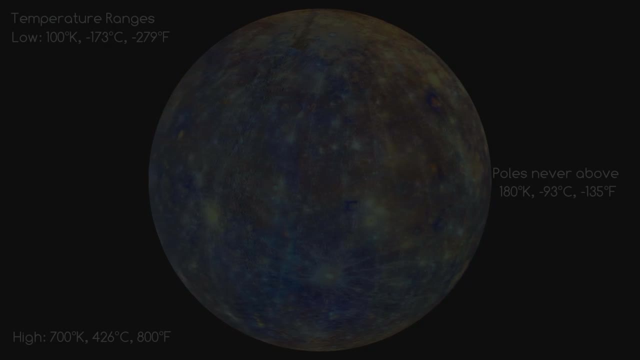 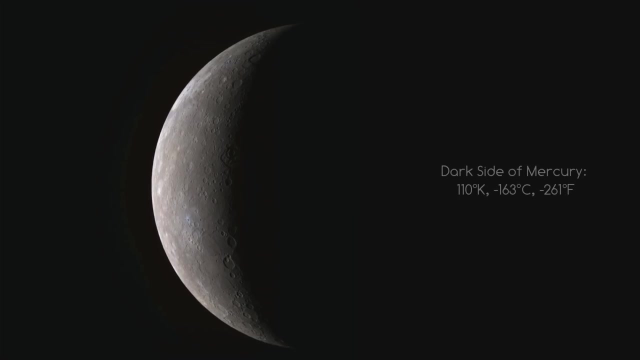 variation is also due to its orbit and rotation, which we will get back to later. The sub-solar point reaches about 400 degrees, while on the dark side of the planet the temperatures are, on average, minus 163 degrees Celsius. This means that the temperature on the dark side of the planet is, on average, minus 163. 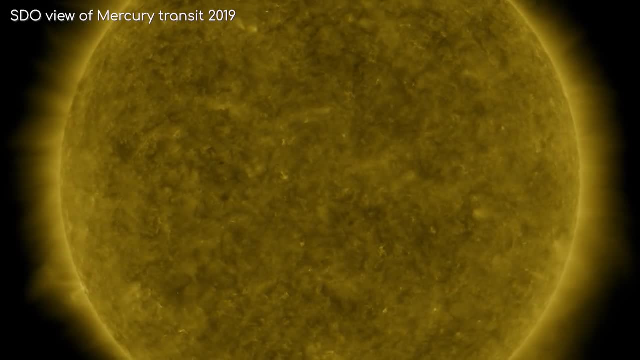 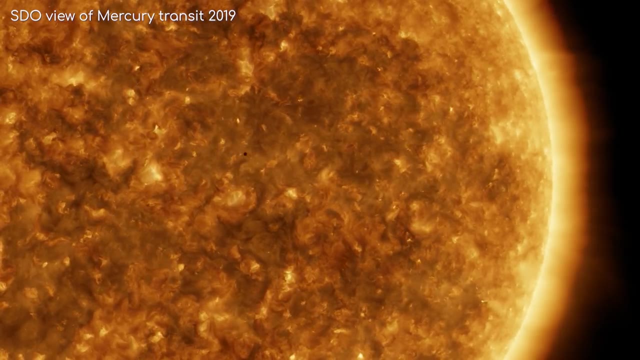 degrees Celsius, Because Mercury is too small and hot for its gravity to retain any significant atmosphere over long periods of time. it's not able to retain any of the heat it gets from being so close to the Sun, which is why the dark side of the planet is so much colder than 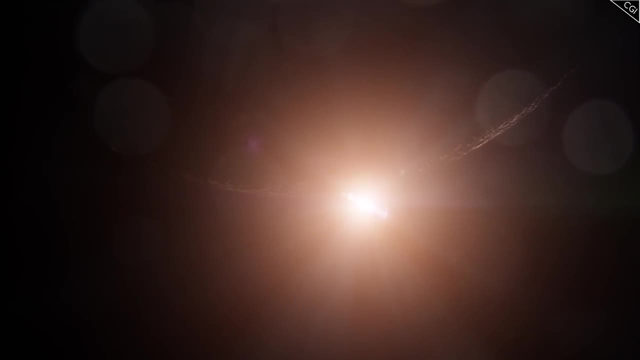 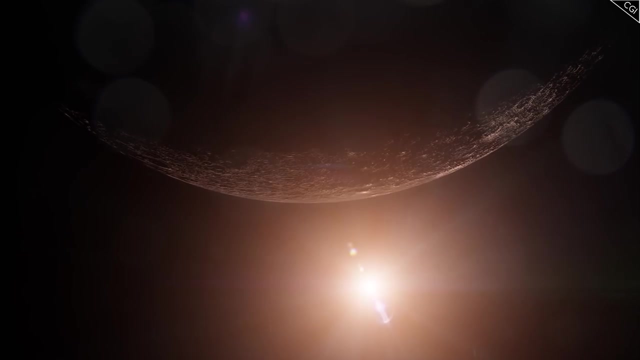 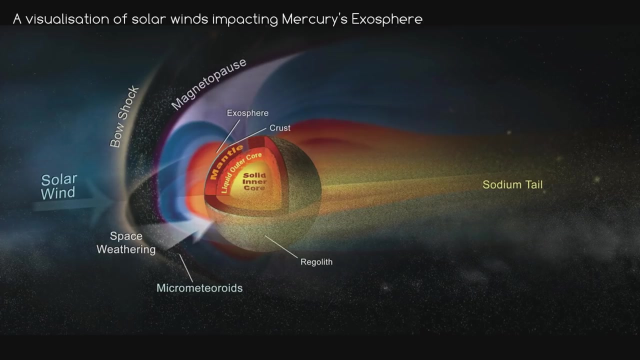 the side facing the Sun. Mercury, however, does have an exosphere, which is like an extremely thin atmospheric-like volume surrounding the planet. Molecules in an exosphere are gravitationally bound to a planet, But the density is so low that it can't behave like a gas because the molecules don't. 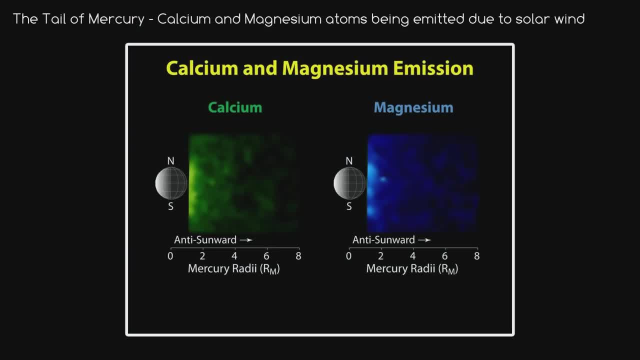 collide with each other. In this picture you can see the messenger probe's view of Mercury's exosphere. When solar wind hits the planet, it rips off certain atoms out of the exosphere and what's left is this trail of atoms going into space. 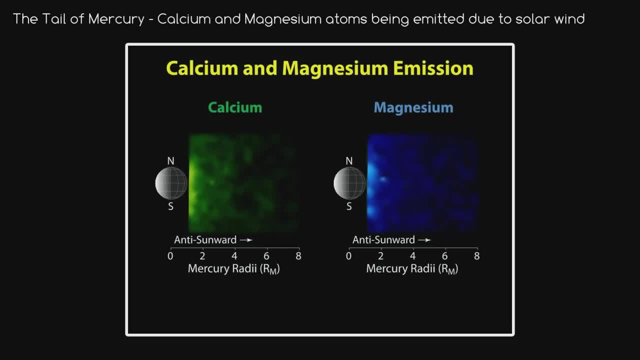 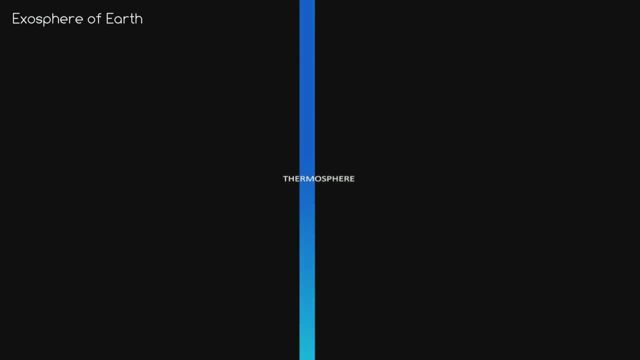 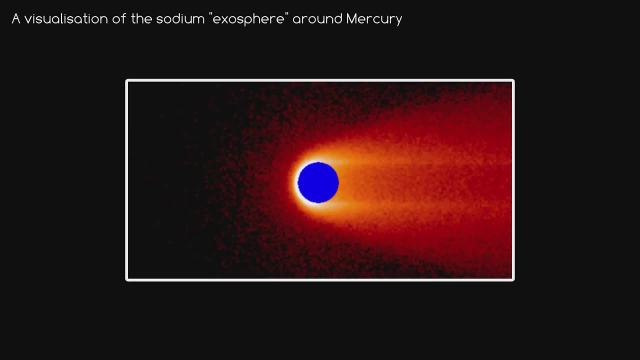 We call this the planet's tail, and every planet has this to a certain extent. Earth even does have an exosphere, But it starts at 600km above the surface. it's really the point where space and the atmosphere meet. Now, in the case of Mercury, this exosphere is not at all stable. 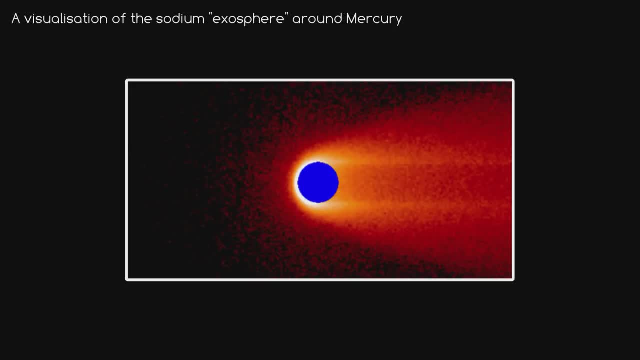 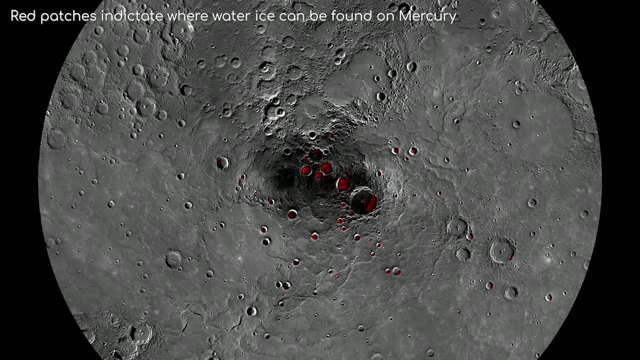 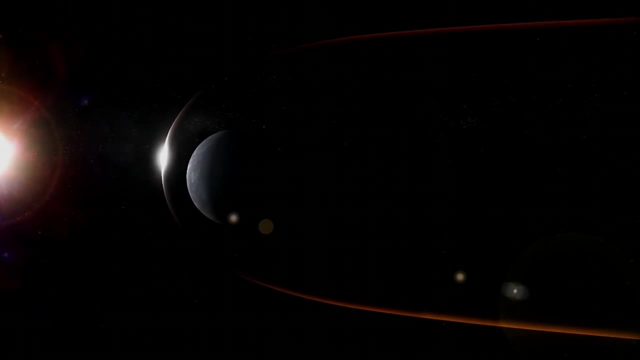 Atoms are continuously lost and replenished from a variety of sources. NASA has been able to confirm that craters at the north pole of Mercury contain water ice. Mercury also has something which Mars lacks: An actual magnetosphere Or a magnetic field all around the planet. 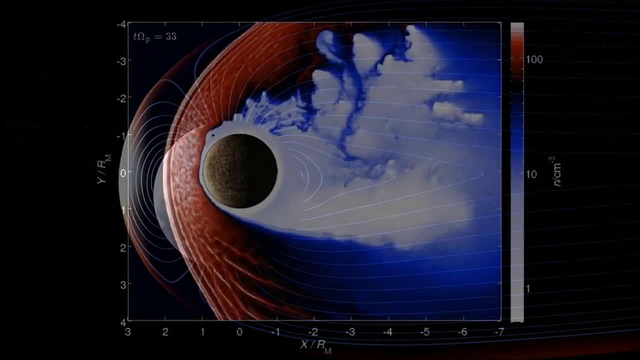 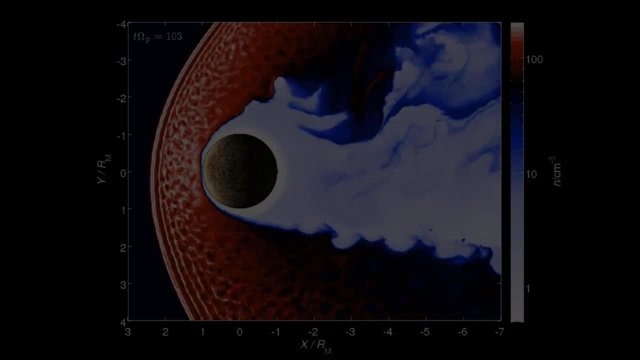 It is only about 1.1% as strong as Earth's, but it's still strong enough to deflect a lot of the solar wind around the planet. Now we're going to get to one of the things I find the most interesting about Mercury. 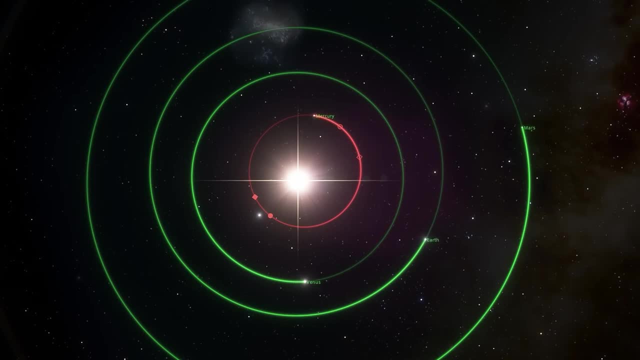 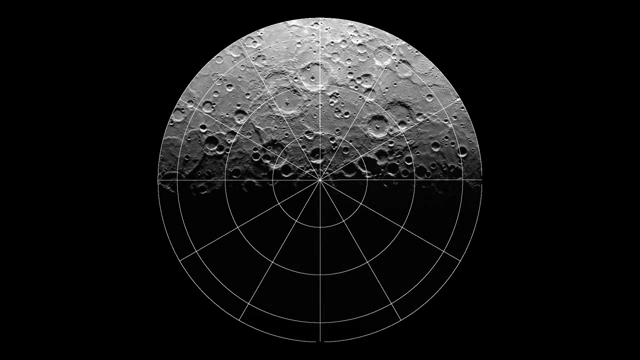 its orbit and its rotation. Mercury has the most eccentric orbit of all the planets, with a distance from the Sun ranging from 46 km to 70 km. Now, this is something a bit hard to imagine, but bear with me. Mercury takes about 88 Earth days to complete an orbit around the Sun. It also has a 3-2 spin orbit: resonance of the planet's rotation around its axis. This means it spins 3 times around its axis for every 2 times that it orbits around the Sun. So, although it takes about 50 km to complete an orbit around the Sun, it also has a 3-2 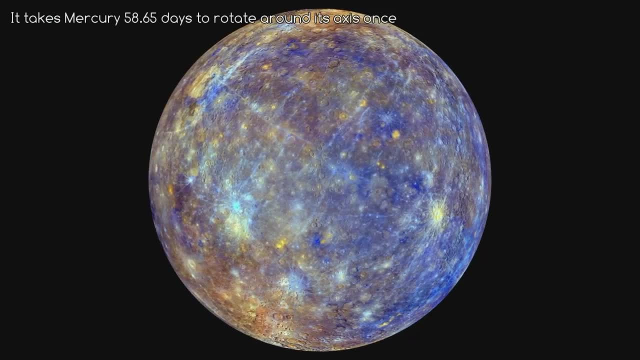 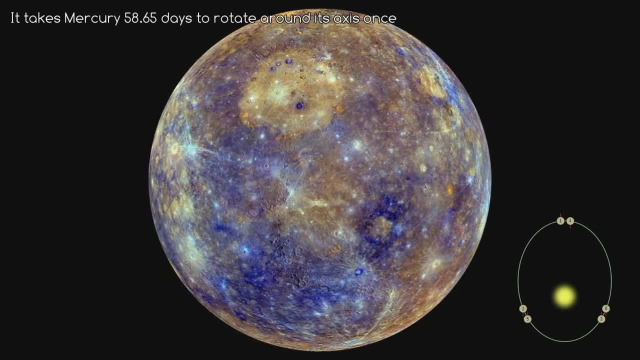 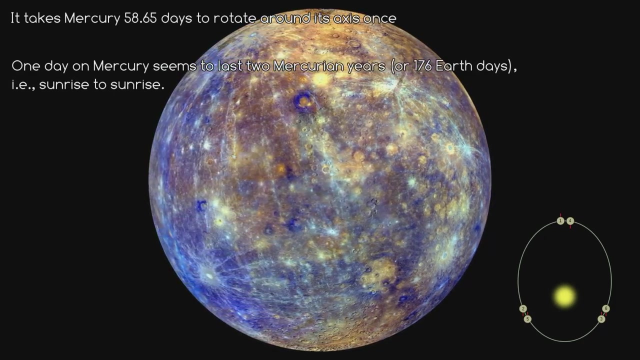 spin orbit resonance of the planet's rotation around its axis for every 2 times that it orbits around the Sun. This means that if you were actually standing on Mercury, it would appear that one day- from sunrise to sunrise, or what is called a solar day- is 2 Mercurian years. 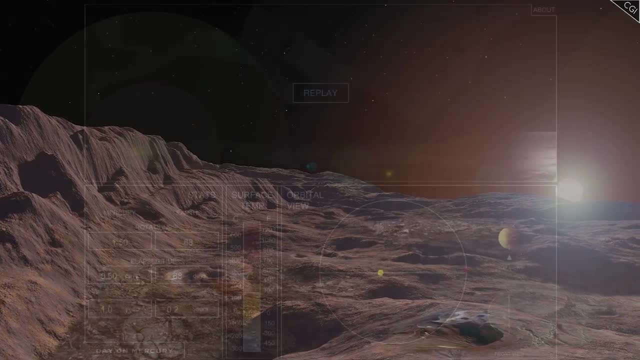 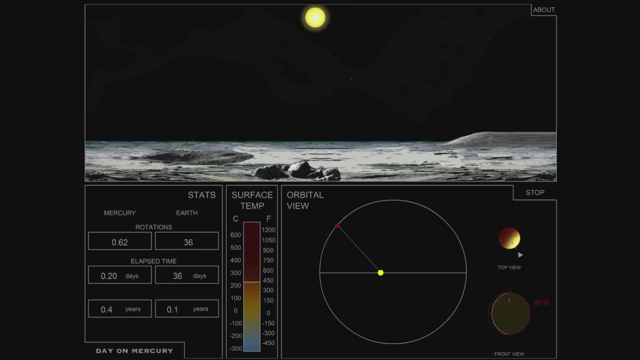 Standing on Mercury, that would look something like this: You would see the Sun rise relatively fast And then, as it approaches midday, it slows down and even starts going backwards, before continuing on again to sunset. As you can see, that took a whole year, which means a night time on Mercury also takes a. 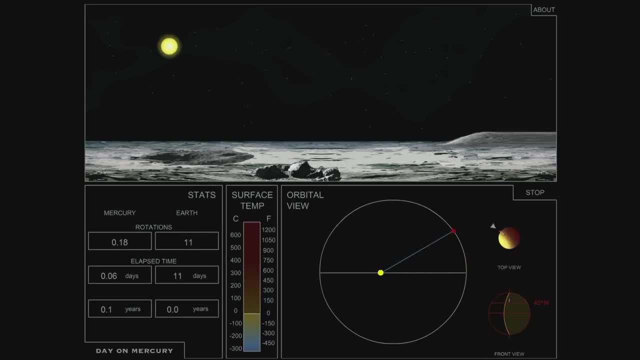 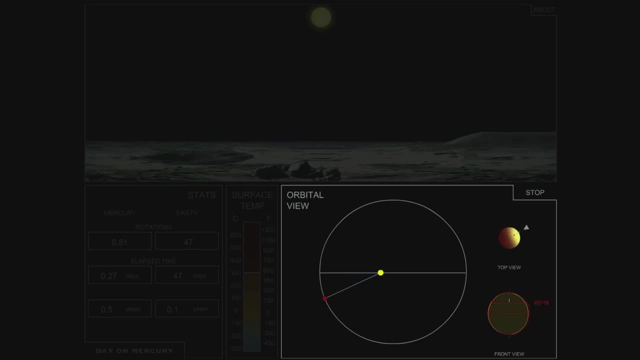 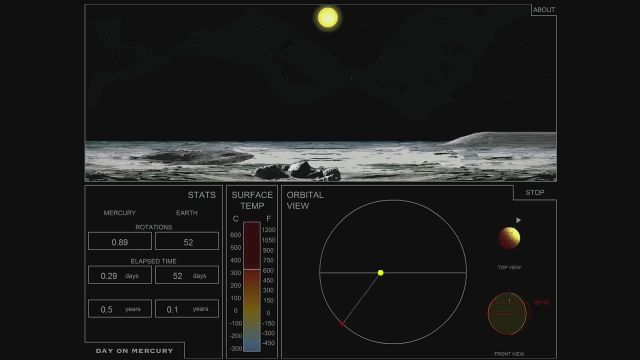 year The Sun starts going backwards in the sky because, approximately 4 Earth days before perihelion, the speed in which Mercury travels along its orbit equals the speed in which it's rotating. At this point, the Sun's apparent motion remains stationary. 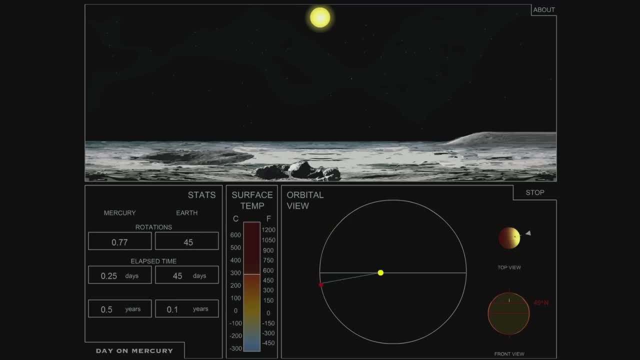 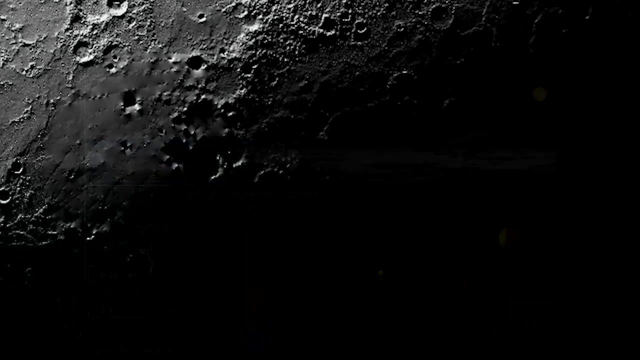 At perihelion itself, Mercury's orbital speed exceeds its rotational speed. So to a person actually standing on Mercury, the Sun appears to move backwards. 4 days after perihelion, the Sun's normal motion resumes. You can see this even clearer from a top-down perspective of Mercury. 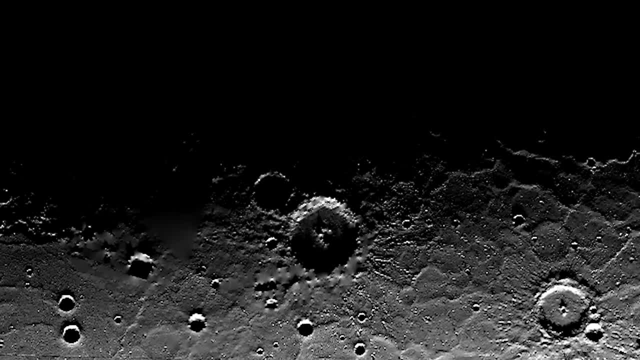 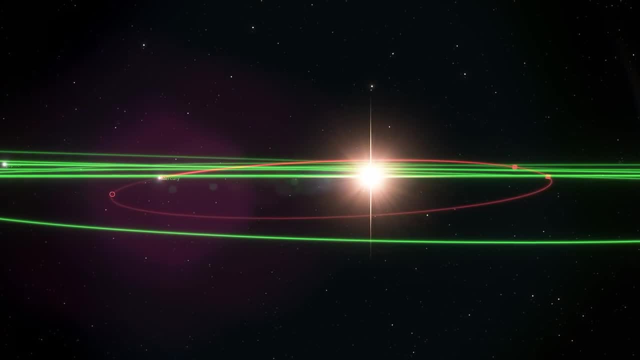 Twice a day. on one of its poles, the Sun seems to pause And then continue on, continue on again. Something else to notice about Mercury's orbit is that it's inclined by 7 degrees to the plane of Earth's orbit. 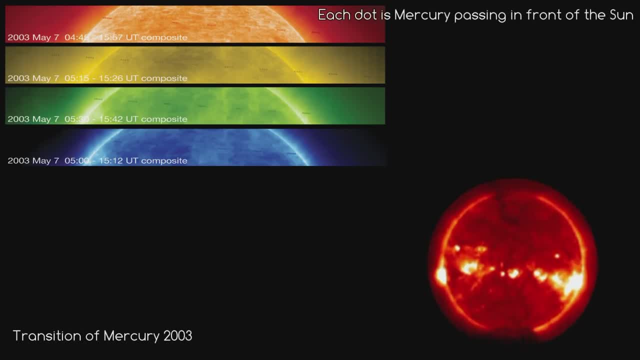 As a result of this, we can only see Mercury transit in front of the Sun when it's directly between us on Earth and the Sun itself, and because its orbit is inclined by 7 degrees. this only happens about once every 7 Earth years. 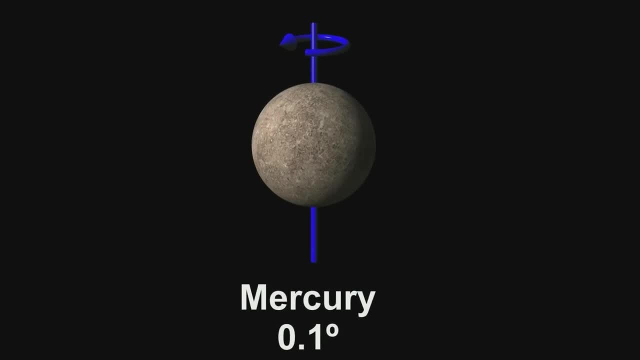 The last thing we'll discuss about the rotation of Mercury is that its axial tilt is almost zero, with the best measured value as low as 0.027 degrees. This is even smaller than that of Jupiter, which has been measured at 3.1 degrees. 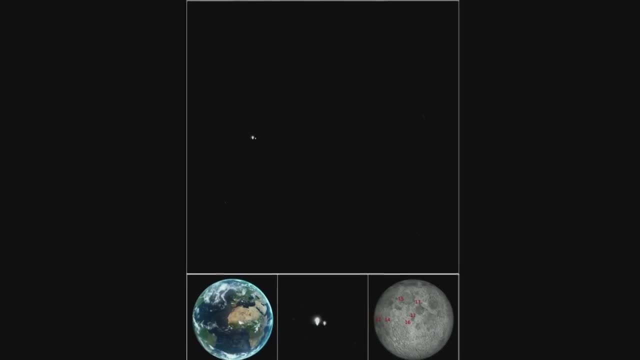 And finally, do you want to see Earth from Mercury Well, here we are, just a couple of pixels across. This photo was taken from the MESSENGER probe several years ago and, barring the newborns, every single one of us was in this picture. 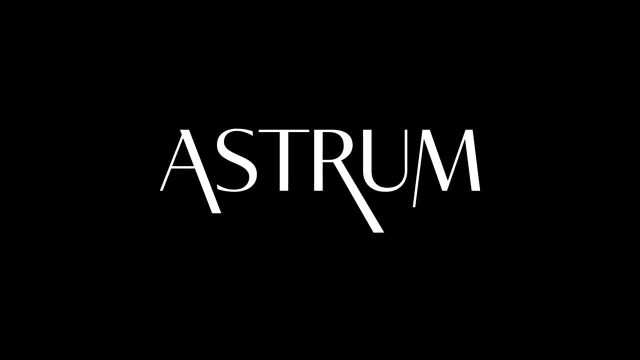 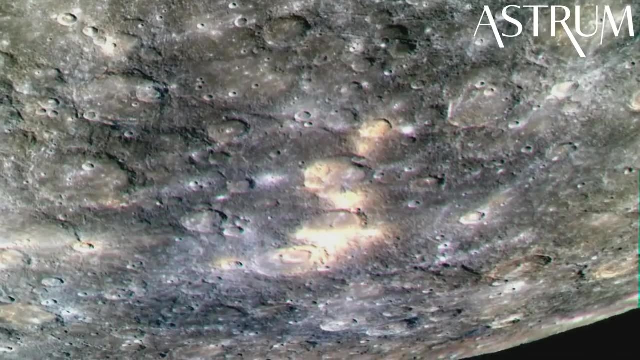 Well, thank you so much for watching this video. I hope you learned something today about Mercury and that it seems more interesting to you now than when you first started this video. If you want to learn more about our solar system, I'm planning on remastering all. 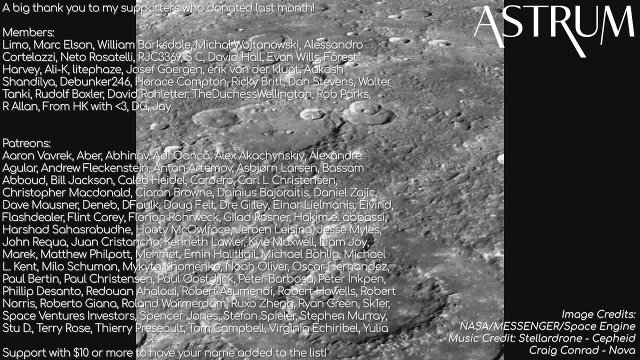 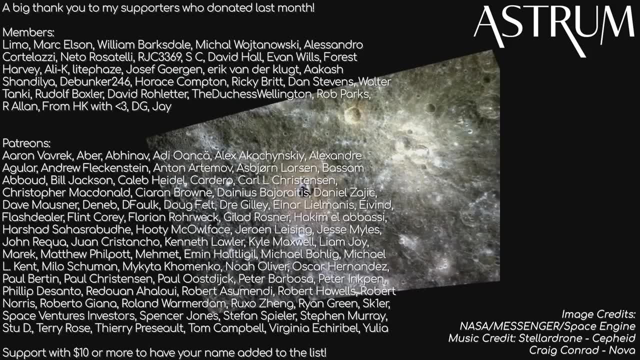 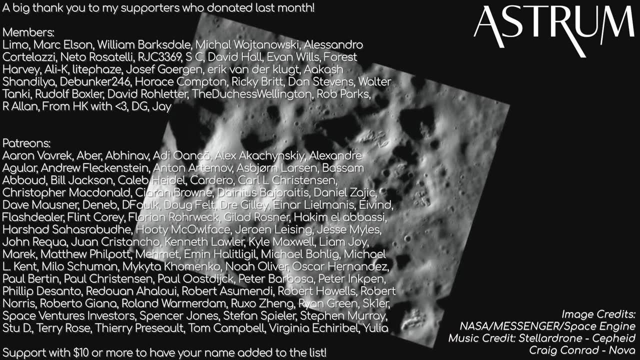 of the old planet videos I've done in the past to bring them up to the quality of my channel currently Find them in this playlist here. The original videos in the series had been a part of the flagship playlist of my channel for a long time. however, the audio quality hasn't aged that well. 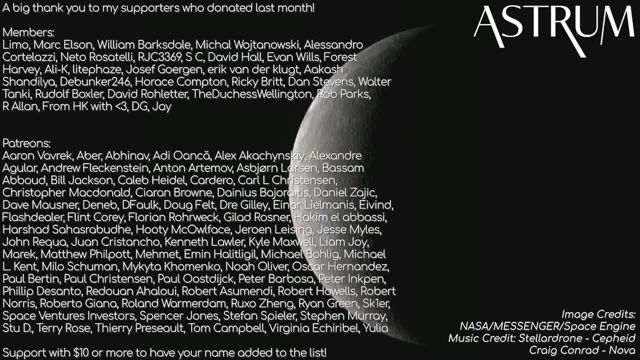 Hopefully now people will be able to enjoy them for years to come. All the best and see you next time. 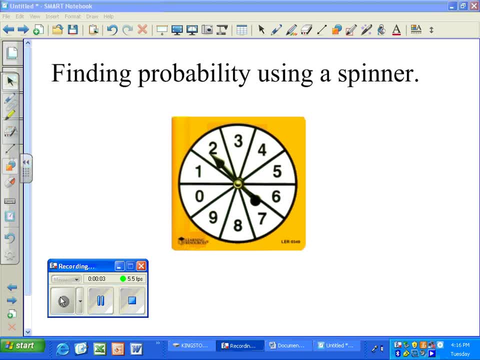 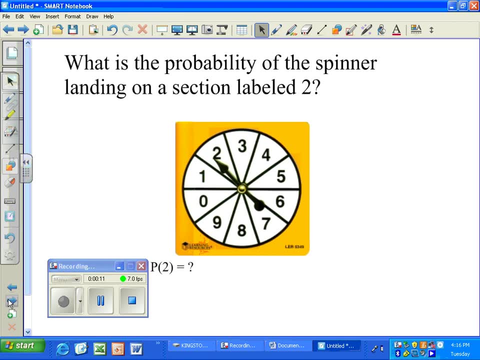 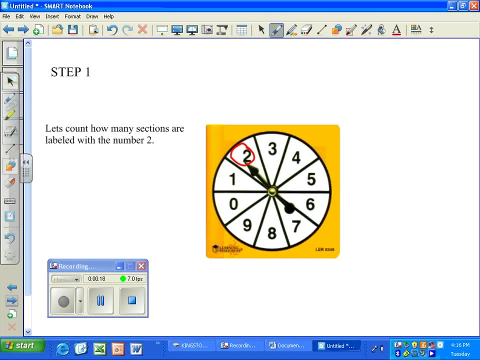 Today we're finding the probability using a spinner. What is the probability of the spinner landing on a section labeled 2?? Step 1. Let's count how many sections are labeled with the number 2.. There is one section labeled with the number 2.. 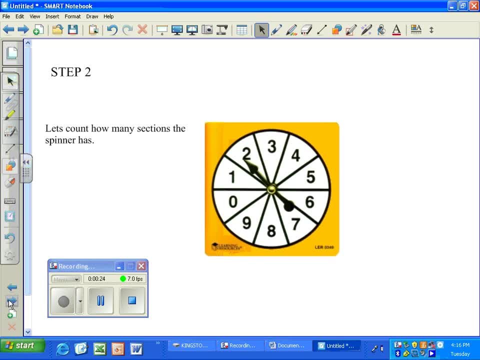 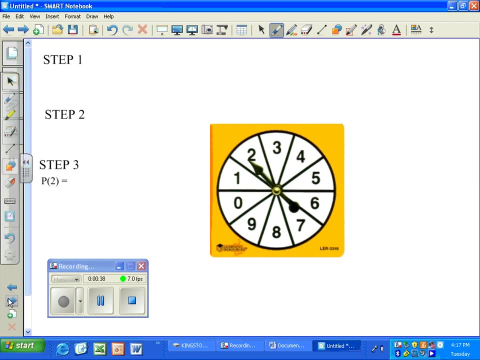 Step 2.. Let's count how many sections the spinner has: 1,, 2,, 3,, 4,, 5,, 6,, 7,, 8,, 9,, 10.. The spinner has 10 sections. 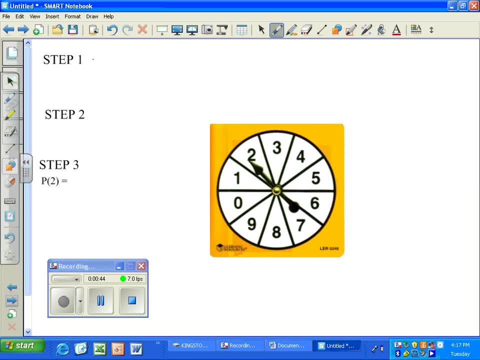 In Step 1, we found that there was one section labeled 2,, so that 1 becomes our numerator. In Step 2, we found there were 10 sections on the spinner, so that 10 becomes our denominator. The probability of landing on the spinner is 10.. 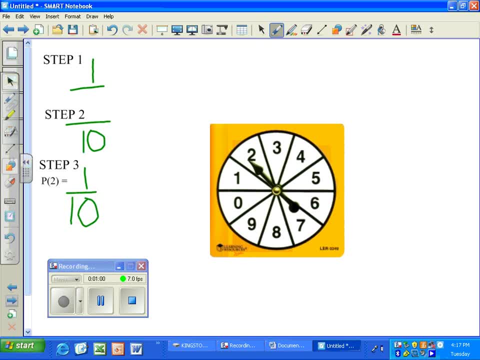 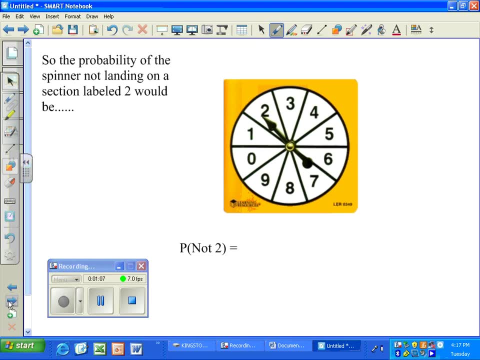 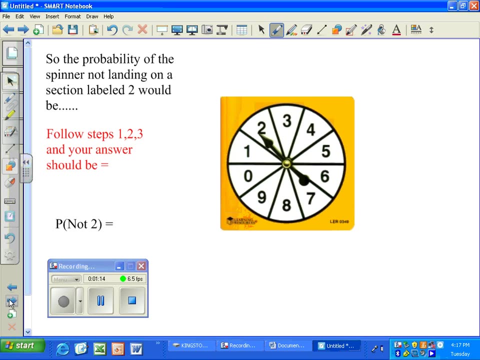 The number 2 is 1 out of 10.. Let's try another one. The probability of the spinner not landing on a section labeled 2 would be: Follow steps 1,, 2, and 3, and your answer should be: